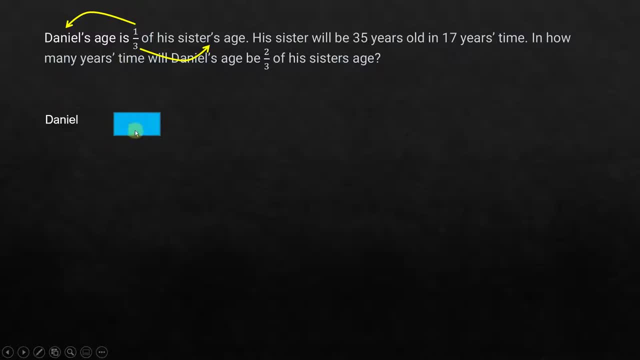 So now let's draw a picture. Let us give a model for Daniel. first, Daniel is 1 part, So sister obviously would have 3 units or parts in his age family. Next statement states he will be 35 in his 17 years time. 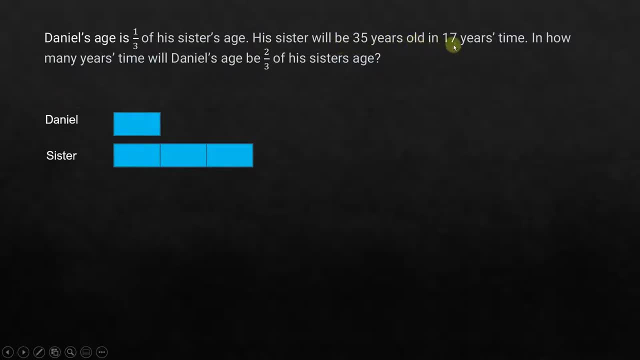 Let's draw another picture and see his age happening. Next explaination says we have the relationship of their ages. with 14th pancake, He is still 2 years. with this age, in another 17 years time- right, her age would become 35 years old. 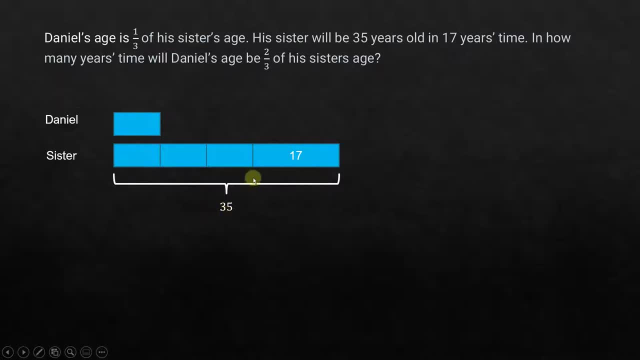 she will be. the total age for her will be 35 years old, after addition of 17 years. of course. at the same time, Daniel will. Daniel's age will also increase by 17, but that is not relevant for us, so we are not doing anything there now when we 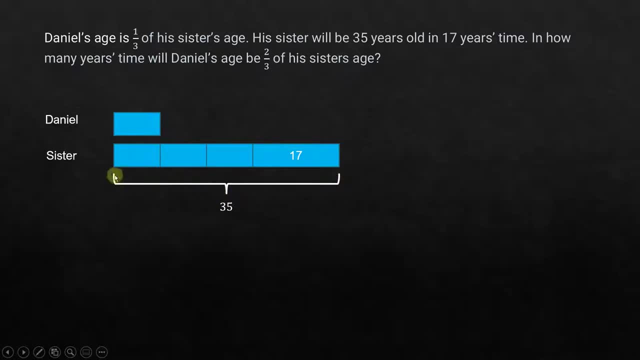 look at this, we find that this whole size is 35 years and out of that- this is a known quantity- 17, which means 35 minus 17, should give us the value of the 3 equal sized units. so 3 units is 35 minus 17, which is 18. 3 units is 18, so we know. 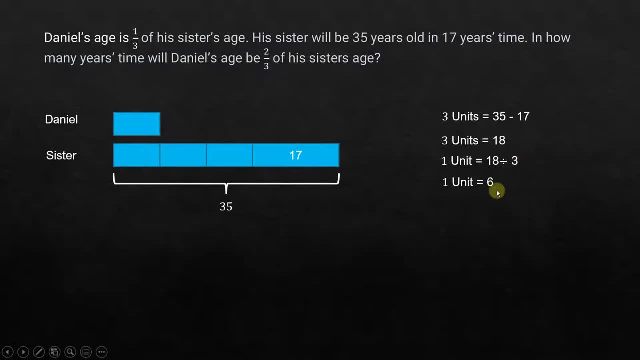 1 year is 1 unit and 1 year is 18, so that's 35 years and that's 35 years, so unit is 18 divided by 3 and one unit is 6.. So now that we know one unit is 6, this one unit refers: 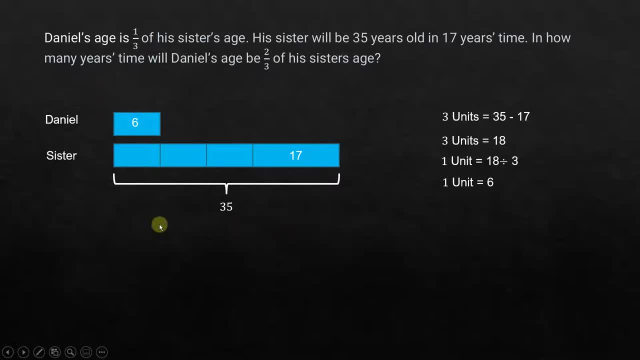 to each of these units here. So each of these are 6.. So that means the current age of Daniel is 6 and the current age of sister- because we cannot include this 17, it's hypothetically saying after 17 years. So currently she's 6 plus 6 plus 6, 8, 3, 6, 18 years old. All right, so we can remove this. 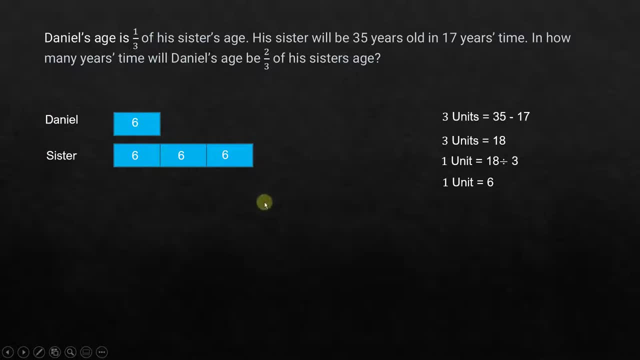 and this because this is the current age that we know of Now. in how many years time will Daniel's age be two-third of his sister's age? Before we go there, first let's look at what is the difference in age between Daniel and sister. 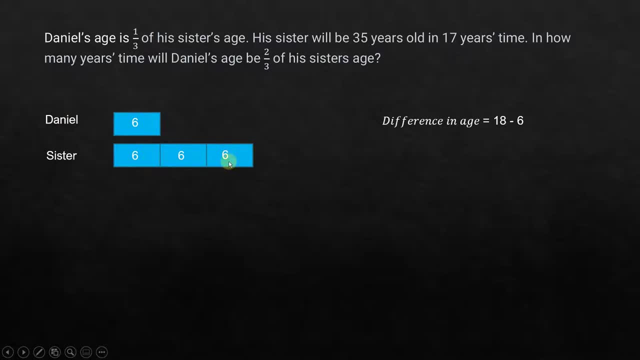 From this it's clear that at 6 plus 6- 12 years, sister is 12 years older than Daniel. and will this difference change over time? No, because every time sister gains one year of age, Daniel will also advance one year in age, which means the difference in age would always remains the same. So in this 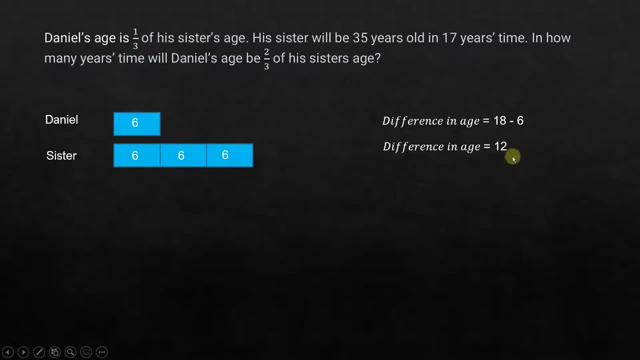 case 18 minus 6, that is, 12 years older than Daniel. Now let's look at the difference between this difference in age. The difference in age is 12.. Now we go to the second part of the question. In how many years time will Daniel's age be two-third of his sister's age? 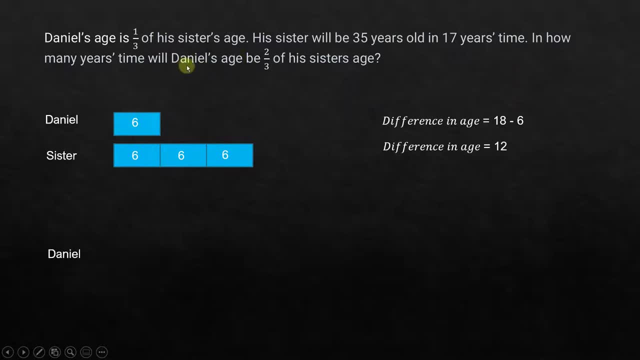 We use the same thing. First, let's just focus on when Daniel's age is two-third of his sister's age, Meaning that, just like what we saw here, Daniel's age will be 2 units for Daniel and 3 units for sister. Daniel's age will be 2 units for Daniel and 3 units for sister. 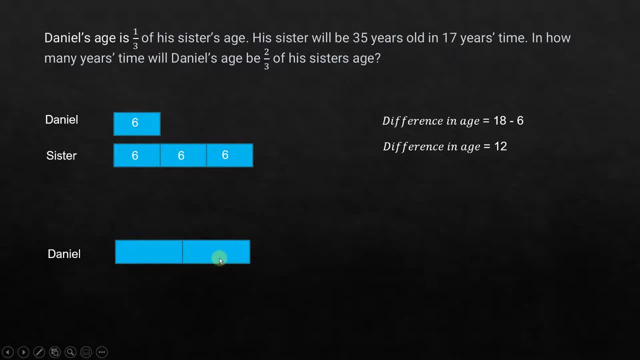 for sister, so Daniel's age. we are drawing two units. remember the unit sizes will may not be the same as this because we don't know the value of this, so we are drawing some other size units- two units and her sister's age is represented by three units. all right, so that's how we represent them here now. 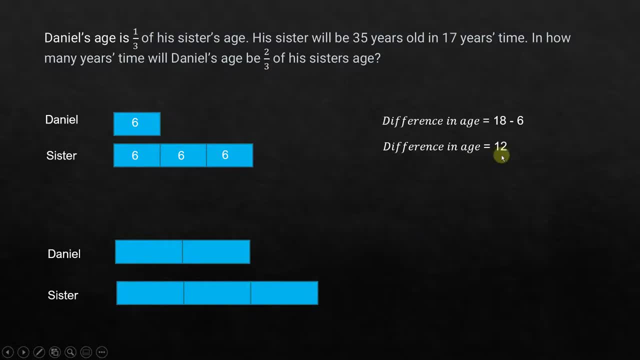 the difference in age that you see here is 12, and that 12 even after many years. the difference between Daniel and sister sage would still remain 12. right after some years, Daniel's age has become two out of three of his sister's age, but we know that the difference would remain 12 years, since we know the difference is. 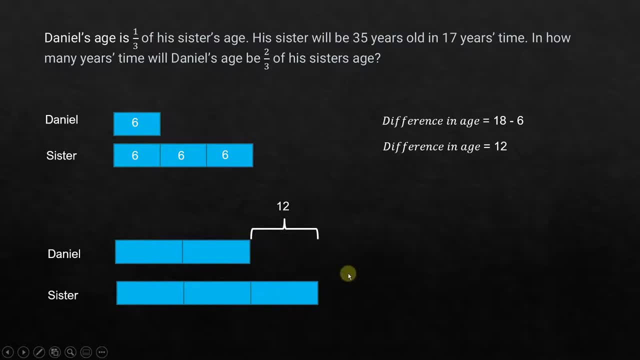 12 years your. so this one unit is going to be 12 years and this one unit is going to be 10 years. so even after many years, if we years, which means these units will also be 12 years, or 12 represent 12.. So at this point of time, 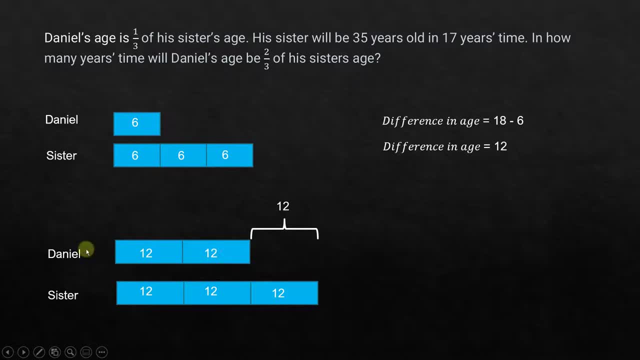 at the time when Daniel's age becomes two-third of a sister's age, what is Daniel's age? Daniel's age is 12 plus 12, 24, right? Currently Daniel's age is 6, and at the time when Daniel's age is going to be two over three times her sister's age, that time Daniel's age would be 24.. So in 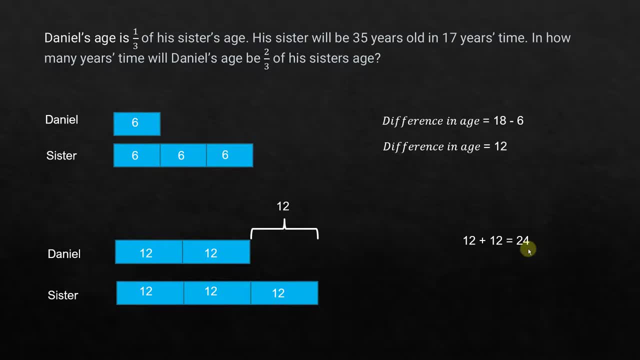 how many years time will he be 24 years old? Now he is six years old, so to become 24 years old, 24 minus 6 is 18.. So in 18 years time, Daniel's age will be two-thirds of his sister's age. 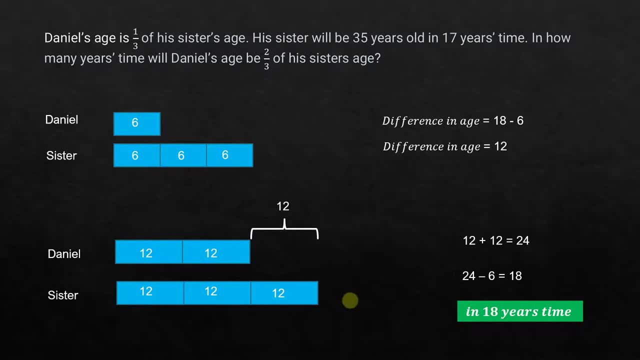 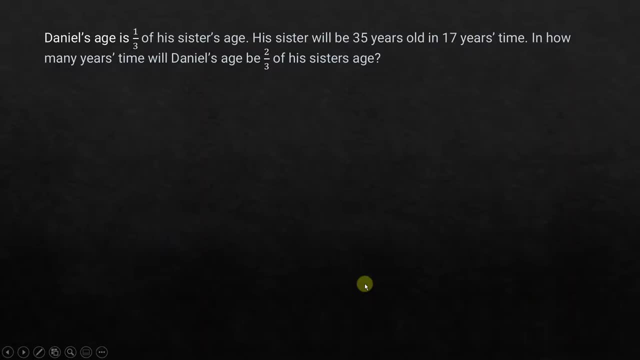 I hope this was clear. So now let's move on to solve the same problem in using algebra. So Daniel's age is one-third of his sister's age. I can assume Daniel age as X and then his sister's age as 3x or three times- Another way of looking at this- Daniel's age is one-third of his sister's. 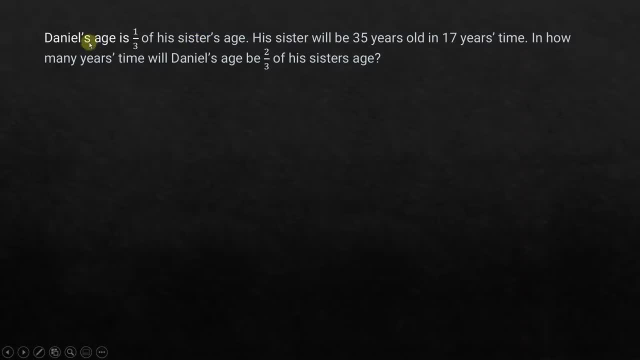 age. Sister's age is three times that of Daniel's age. That is another way of looking at it. So let's say Daniel's age is X, then Daniel's sister's age is going to be 3x And his sister will be 35 years. 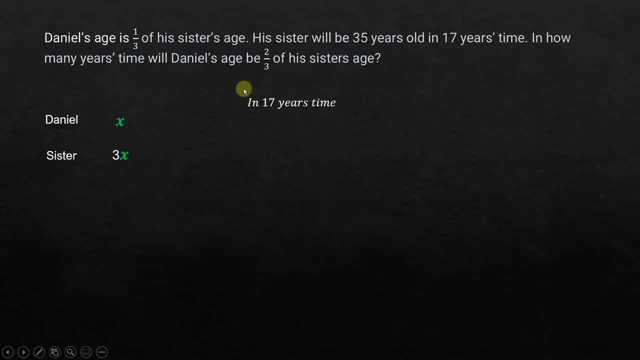 old in 17 years time. In 17 years time, what will be her sister's, Daniel's sister's age? Right now, Daniel's age is 3x. In 17 years time, it should become 3x plus 17.. Right, But we know the actual. 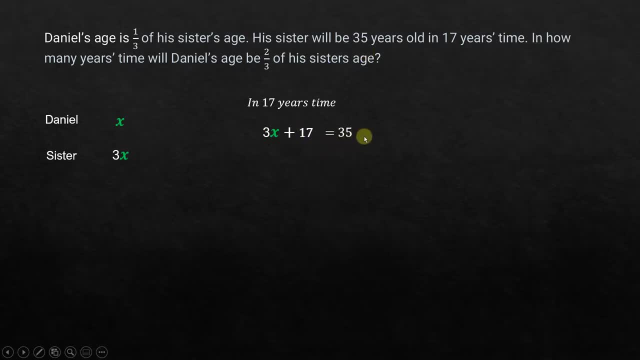 value of her age, which is 35 years old. so this should be equal to 35.. So this gives us an equation to solve and find the value of X. So 3x is 35 minus 17 and that is equal to 18.. So X is 18 divided. by 3, which is 6.. So now we know that 3x is equal to 35 years old. So now we have to solve the same problem. So we have to find the value of X. So 3x equals 18.. So x is 18 times 3, which is 6.. So now we know that 3x is. 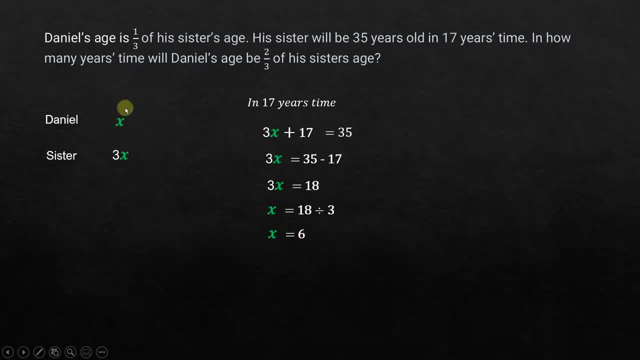 x is 6, which means Daniel's age is x, which means it is 6, and Daniel's sister's age is 3 times x or 3 times 6, so it's going to be 18.. Daniel's age is so in this case. in how many years time? 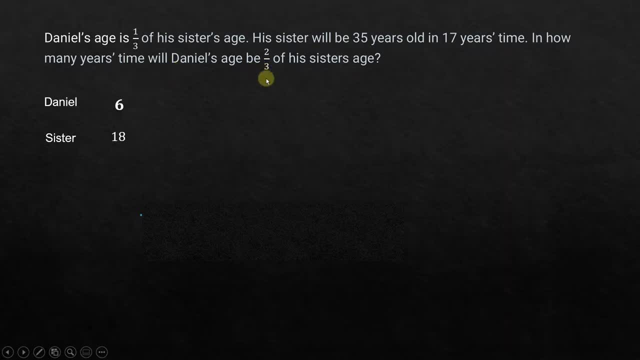 will Daniel's age be 2 3rd of his sister's age. so that is what we are going to figure out. so difference in age, we know is 12, so the difference in age does not change over time. so that is the concept that we are going to use all right now. now Daniel's age is going to be: 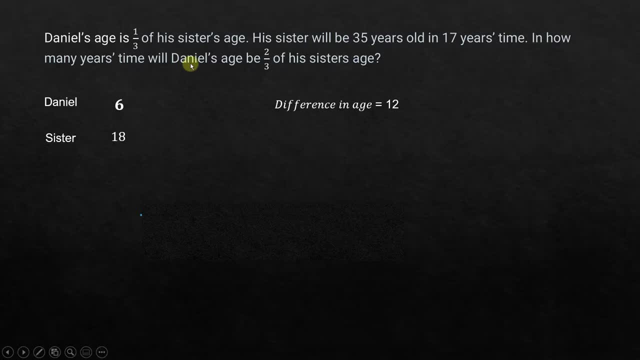 2- 3rd of his sister's age, which means we can represent this as as Daniel's age is 2x and his sister's age is 3x, So sisters, or, in this case, instead of confusing with the previous x that we used, 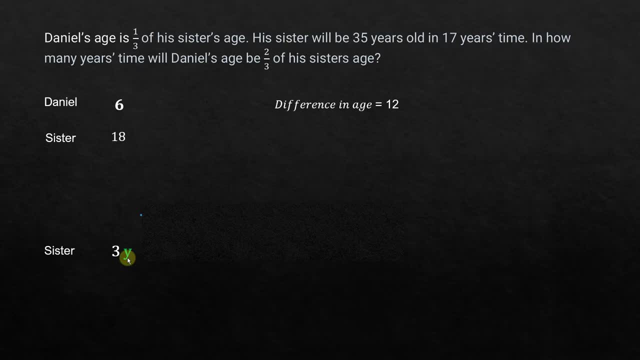 we could use any variable. We could still use x, but just for clarity we are going to use another alphabet, y, here. So let's say sister, this can very well perfectly be used as 3x, but for just clarity. 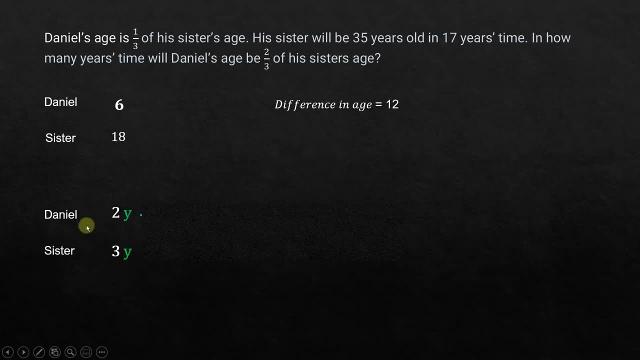 we are just using it as 3y. Sister is 3y and Daniel's age is 2y, all right, So, and we know that the difference in their ages is going to be 12.. So 3y minus 2y is going to be 12, which 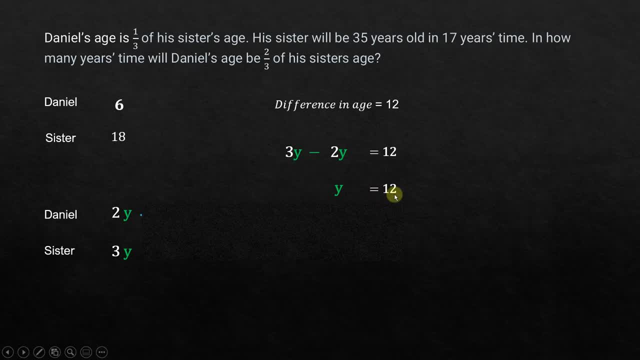 means y is going to be 12.. And since y is 12, we know that Daniel's age is 3y. His age is 2y, which means it's going to be 2 times 12, which is equal to 24.. 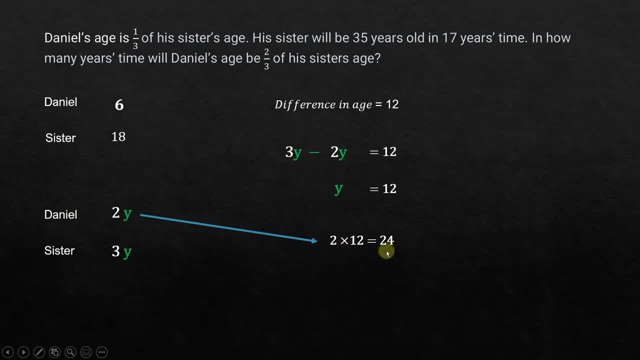 So Daniel's age is 24 when, that is, when his age is 2 thirds of his sister's age. But currently Daniel's age is 6, right, When his age becomes 2 thirds of his sister's age, his age would be 24..